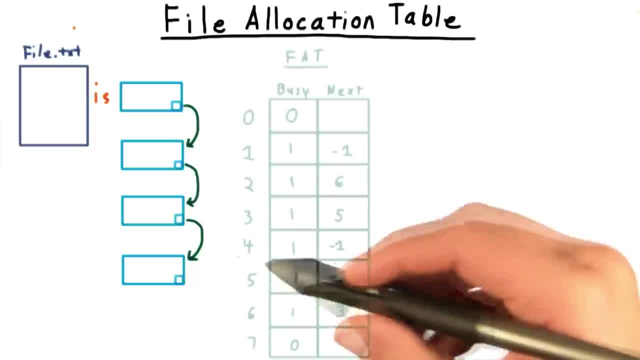 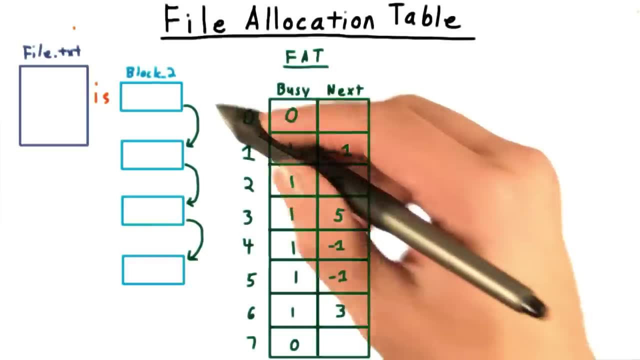 Maybe the last part of the block would give the ID of the next block Here. however, the links in this list are represented in the file allocation table, which is indexed by block number. Giving the starting block number of a file, I can find the next block. 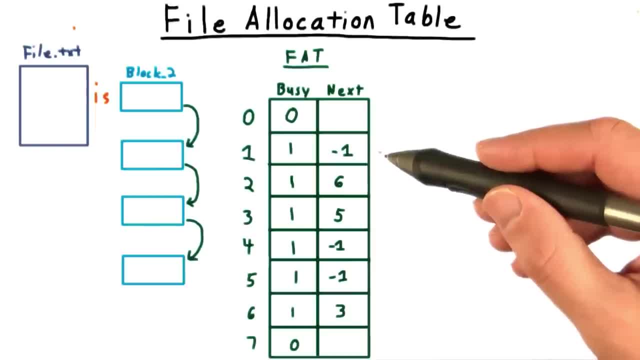 with a constant time access to the file allocation table. A special value, negative 1 in this example indicates that a block is the last in the chain. This file allocation table also contains a bit to say whether a block is free or not. 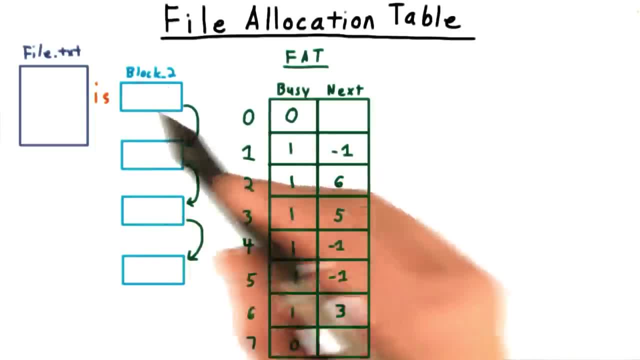 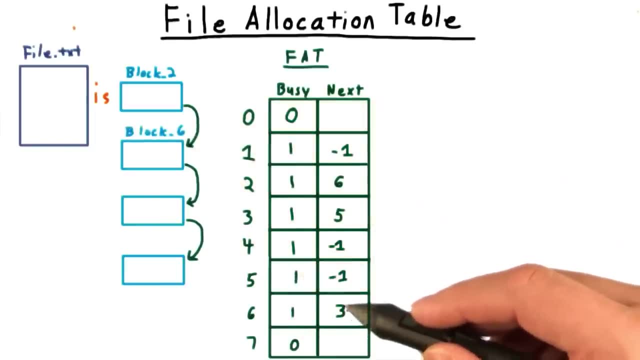 In this example, our file starts with block two. Looking at the table, I see that the next block is six. Looking at six in the table, I see that the next block is three. Again going back to the table, I see that the next block is five. 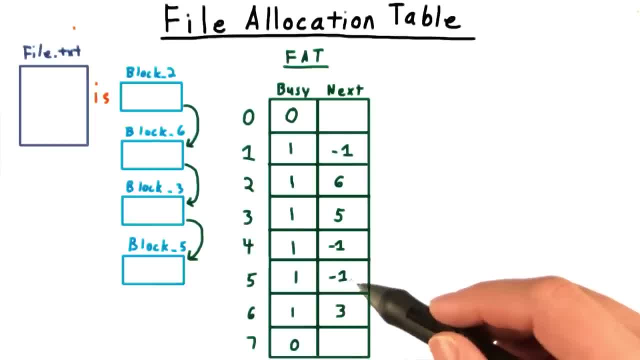 And when I look at five in the table, I see that it's next has the special value indicating that we've reached the end of the file. It's important to realize that the file allocation table- or FAT for short, stores all the links for all the files. 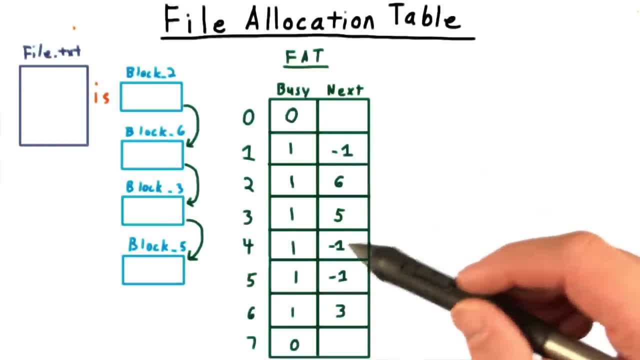 For instance, there appears to be another file occupying block four, and only block four, since that's the end, And also one occupying block one. So the file allocation table tells us how to glue the blocks of a file together, but it doesn't tell us where to start these chains of blocks. 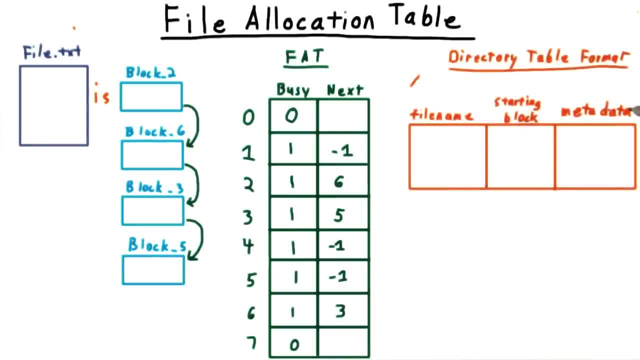 That is the function of the directory tables. Directories, I should say, are indeed treated as files, and they use something called a directory table format. Entries in the table all have the same width and contain the essential information, Including the file name, the starting block and. 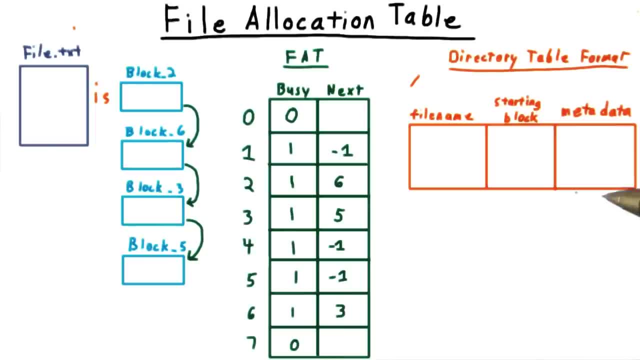 any other metadata associated with the file, such as permissions. The root file directory has a fixed address on the disk, so we always know how to get started. Let's say that I wanted the content of a file slash, foo. slash, file, dot. txt. 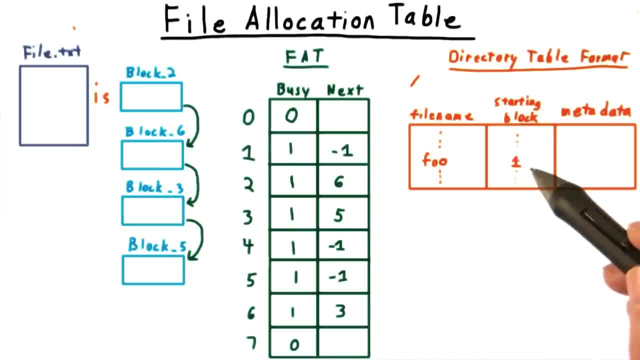 I would first consult this root directory table. It would tell me that there is indeed a directory named foo and give me the starting block of that file. I would then access that file on the disk And, since it's a directory, I would look through there for. 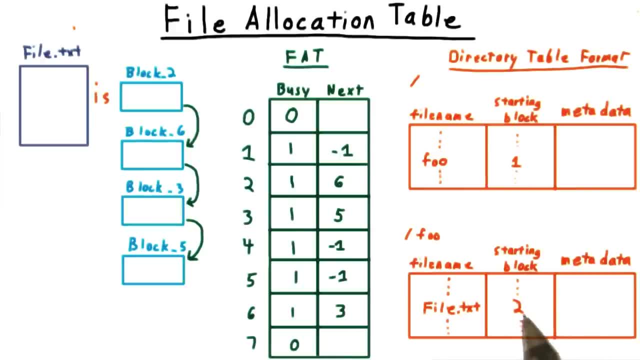 the file name, dot txt, and it would tell me that the starting block is two. I can then chain together the blocks on disk, as we did earlier, using the file allocation table. To summarize then the FAT or file allocation table: 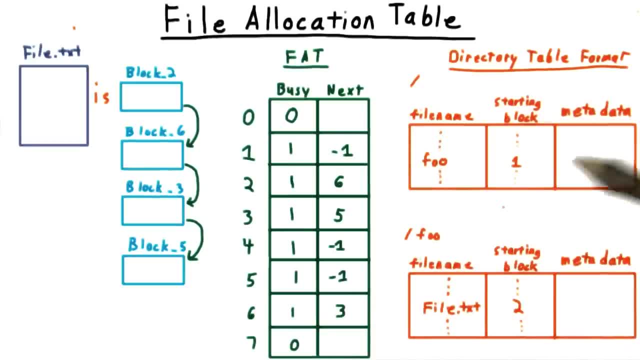 serves as the glue that chains the blocks of a file together. The directory files capture the hierarchy and the starting blocks for the files and all the metadata. 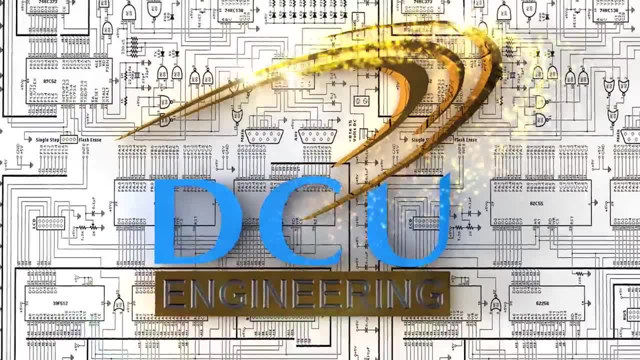 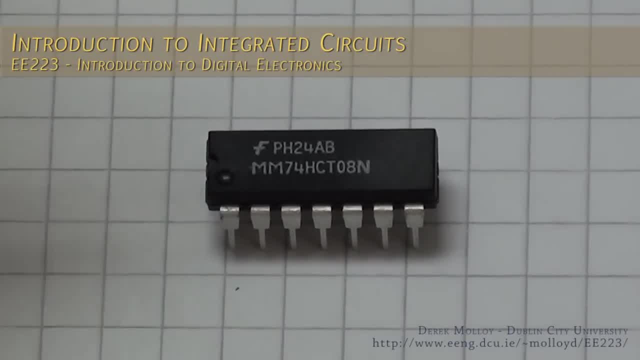 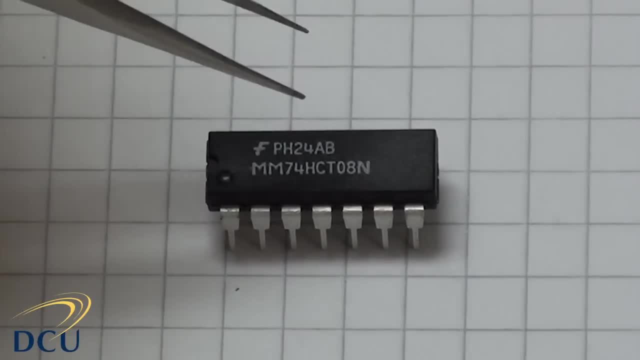 In this experiment we're going to look at integrated circuits and we're going to build some experiments from the course notes and implement them on our breadboards. We're going to first look at the chips themselves. This is the type of chip that we're going to use. 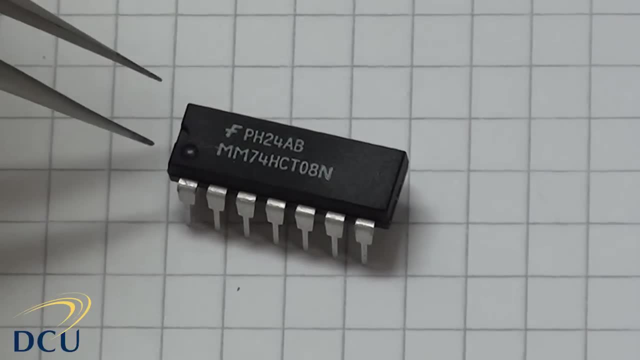 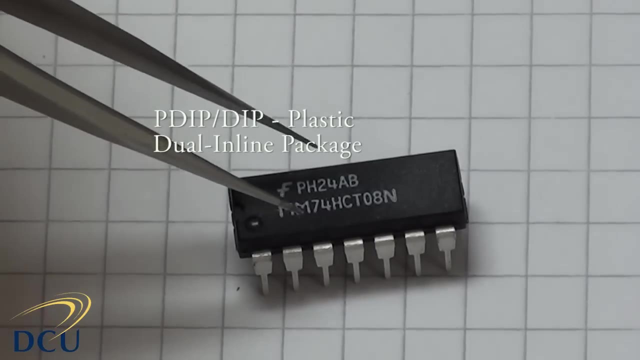 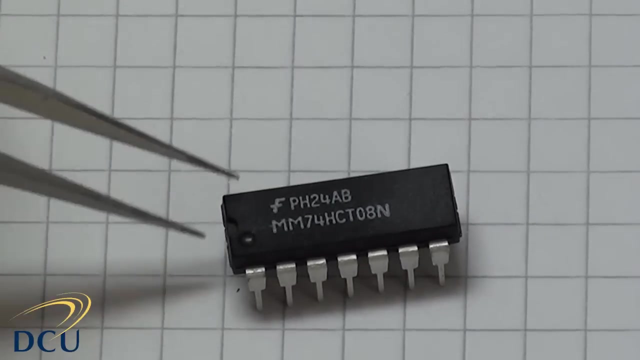 the type of chip packaging we're going to use. It's the DIP packaged chip, which means plastic dual line. the pin package. The pins are spaced at 3 tenths of an inch apart. You can see that you have a little circle here at the very top that indicates that that's. 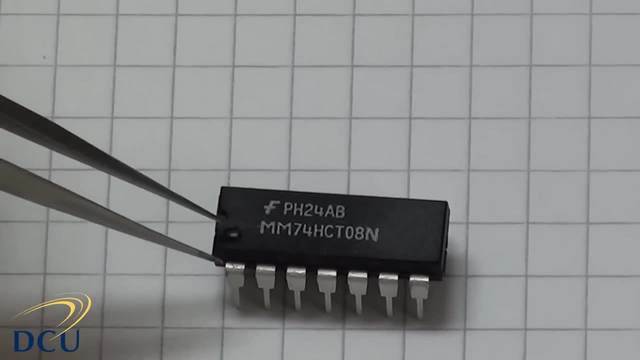 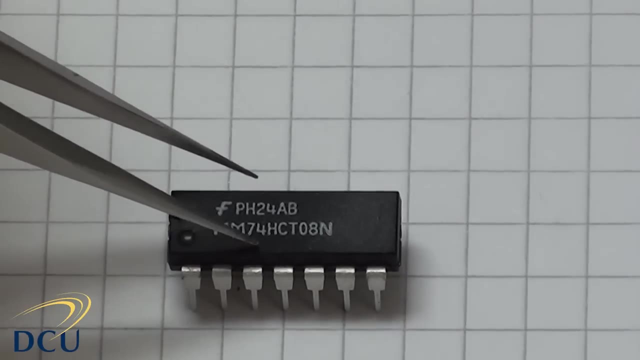